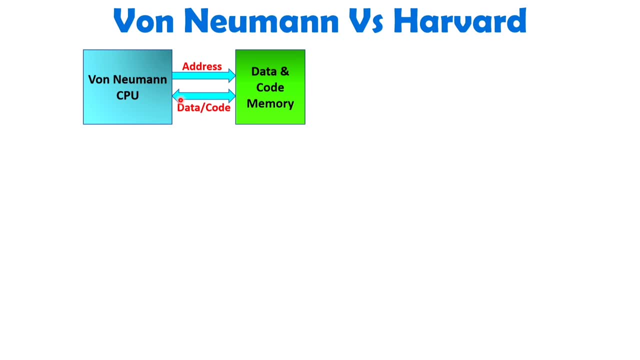 read code from the memory. But when you access data, at that time you may be reading memory as well as you may be writing into the memory, right? So bidirectional data code that is shown over here, right? And when we talk about Howard architecture, at that time you will be observing that for data and for code we have separate memories. So you can observe here, see, with this data memory. 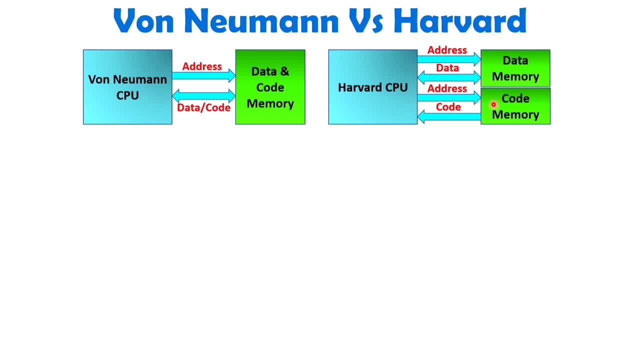 we are having separate address for code memory Also, we are having separate address right, And you see, we are accessing data with bidirectional access, right, And with code. we are just reading data over here And that data will be code. Code means program, right. So with Howard architecture, data memory and code memory are separate right, And addressing is also separate over here. 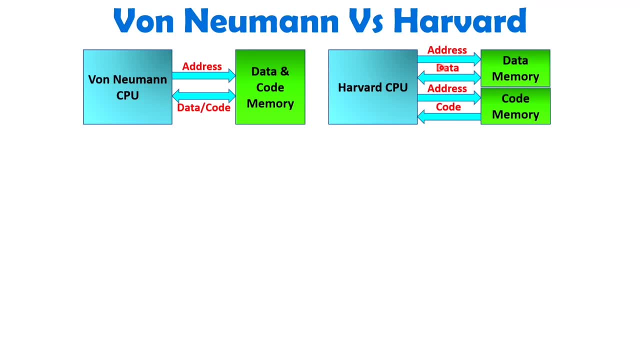 Now, here there are a few essential things that we need to understand and that you can easily understand based on comparison. So here, with respect to different parameters, I'll compare von Neumann and Howard architecture. See, as I have told you, for memory access, you should know data and program are stored in same memory. with von Neumann architecture And with Howard architecture, data and program that is stored with 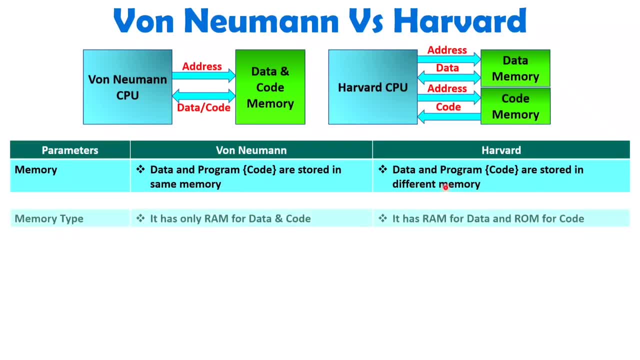 different memories right Here, my dear students, when we talk about memory type, then you should know that here, with von Neumann, data and code memory, that is same right, And here you see code that we are delivered to read, but data access will be bidirectional, in that we will be reading as well as writing data. So common memory should be RAM only right, As we need to perform. 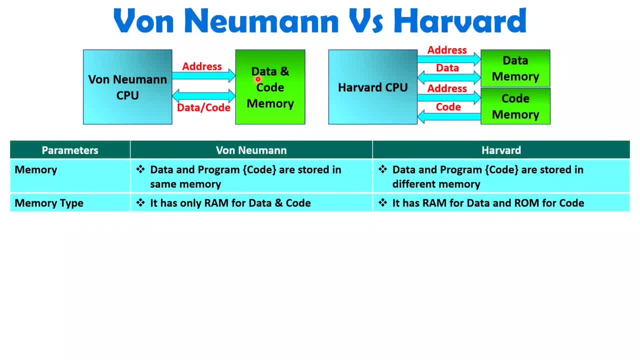 read and write operation with data, this common memory for data and code. that will be RAM. With Howard architecture in data, you will be observing bidirectional data access is happening. Why? The reason is here: we need to read as well as write the data. So for that you need to have RAM with data memory, And for code memory- or you can say for program memory- you just need to read program right inside CPU. So here you. 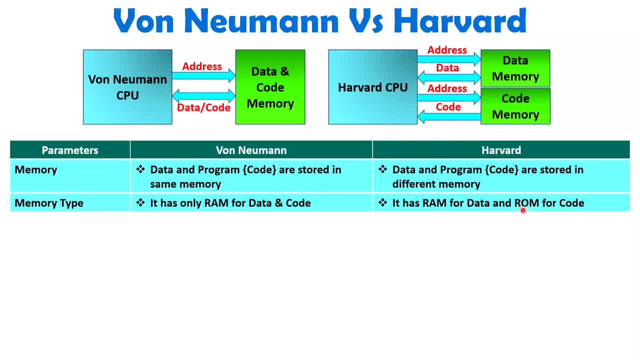 you will be using only ROM. that is read-only memory, right. So that is how different memory types will be there. Now, my dear students, when we talk about buses, then you should know: for data and code access, you will be having common buses for address and data, right. 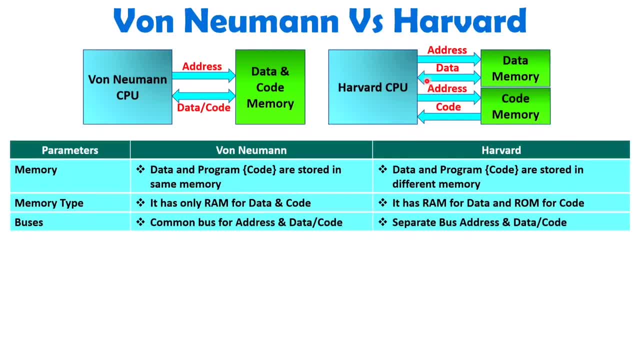 And here, with Harvard architecture, we have separate addressing right, So for data access, addressing is separate And for code access we have separate addressing right, So separate bus will be there for address as well as data with Harvard architecture. 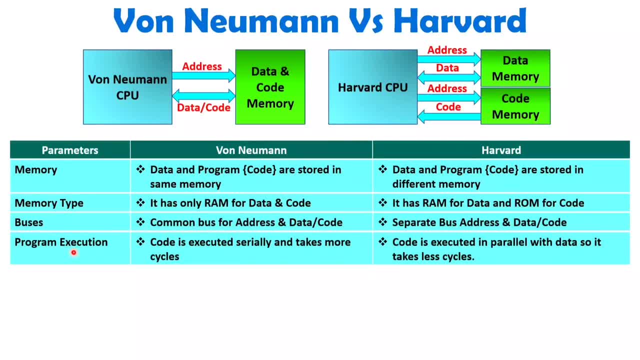 Now, my dear students, as if you see how program execution is happening, then with Von Neumann architecture, here code will get executed serially, right, And here, see, you cannot have parallel execution. First you will be executing code and as if it is having a requirement of data. 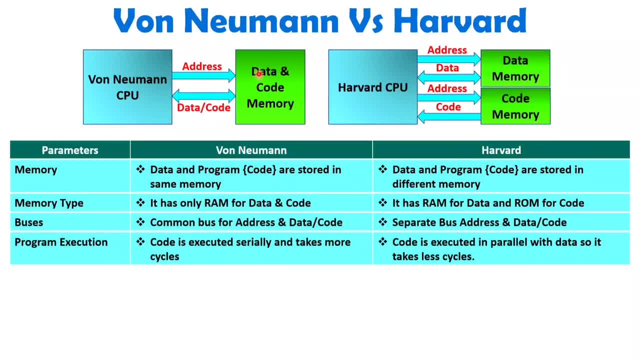 then data will get read and write from same memory, So execution will be serial over here. But with Harvard architecture, you will be observing, execution of code can happen in parallel with data. Why? The reason is we have separate address right. 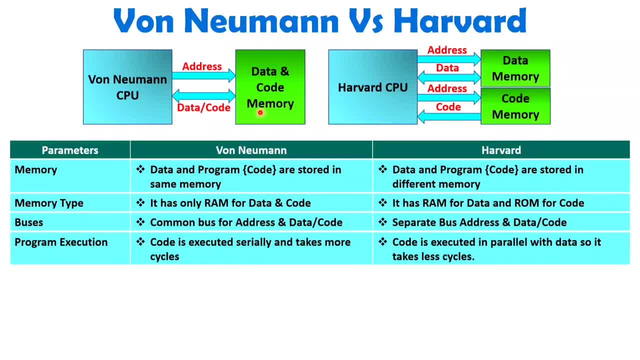 My dear students, you should know that, as if you have any memory in that at a time you can either perform read or write operation, right. But here, with Harvard architecture, we have separate memory for data and code, So we can have parallel execution with code and data. 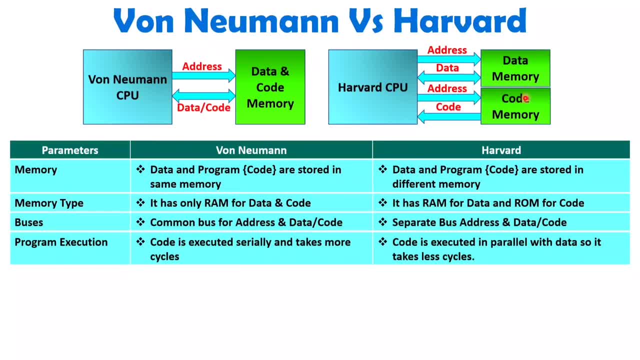 as separate addresses are available for code and data right. So you can say: when you execute program using Von Neumann architecture, you can have parallel execution with code and data, as separate addresses are available for code and data right. So you can say: when you execute program using Von Neumann architecture, 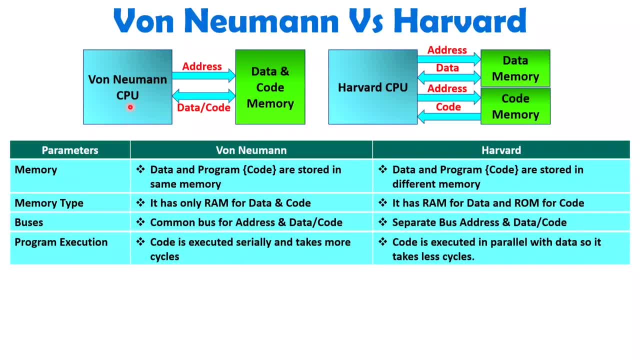 at that time you will have to take more machine cycles for execution of program. But with Harvard architecture you can have parallel access of data and code. So in that you will be taking less machine cycles. Machine cycle means you may be reading the data. 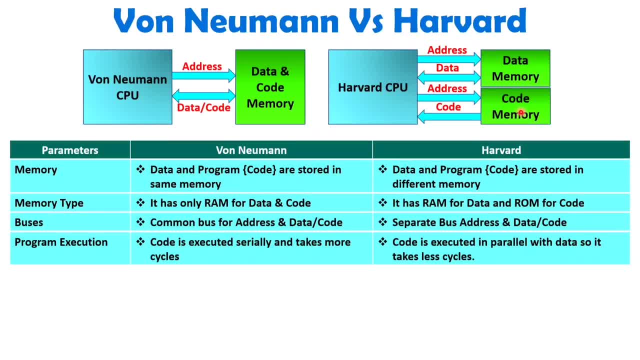 you may be writing the data, you may be fetching the opcode of program, right? So these are the machine cycles which may be there with program. So here, parallel machine cycle execution is possible. Here, my dear students, when we talk about data code transfer, 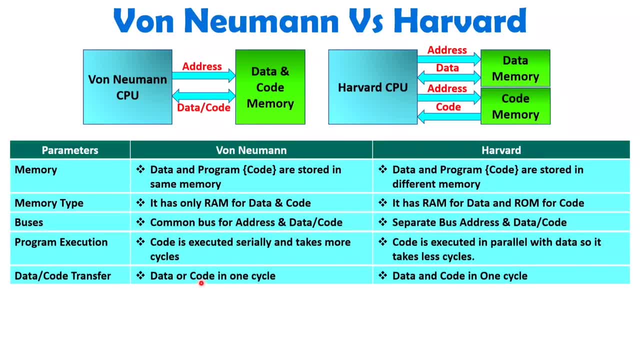 then you can have data transfer or code transfer with single machine cycle. But with Harvard architecture data and code transfer that can happen in one machine cycle only. right, As we have separate addressing with Harvard architecture Here when we talk about control signals. 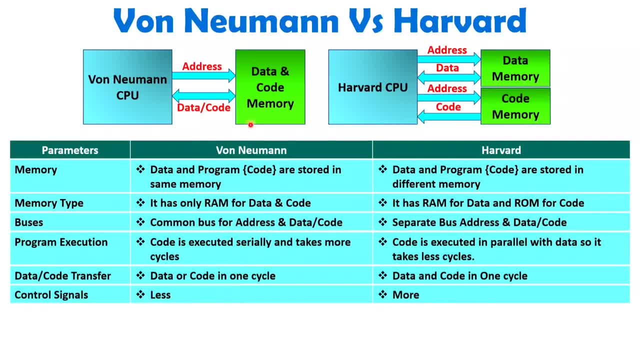 then obviously you need to have less control signals, right, As you have common memory over here. What are those control signals? Those control signals are memory read and memory write, right, And here you will be having more control signals with Harvard architecture. 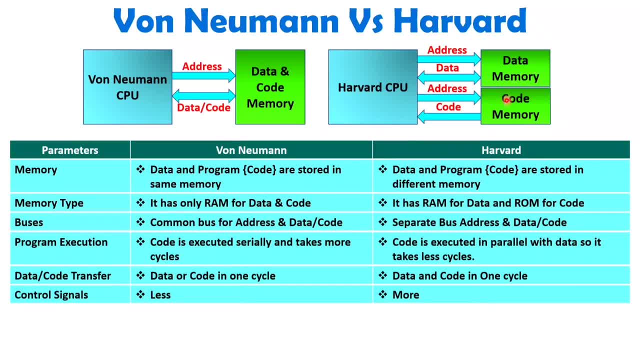 as you have data and code memory with separate addresses, right. So for data memory, you will be having a need of memory read as well as memory write control signals, And for code memory, you will be having a need of memory read control signal. 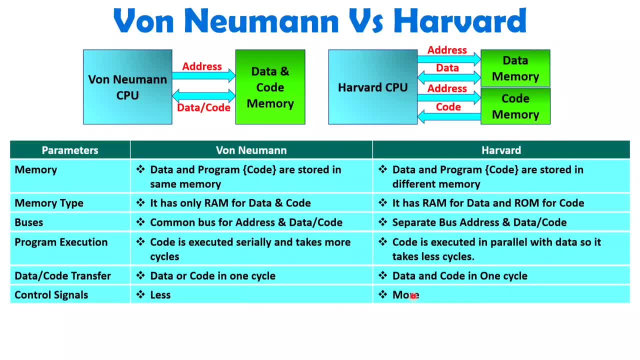 So here you will be having a requirement of more control signals with Harvard architecture. Here, if you see the space requirement, then you will be having a less requirement of space with one Newman. Why? The reason is you have single memory for data and code. 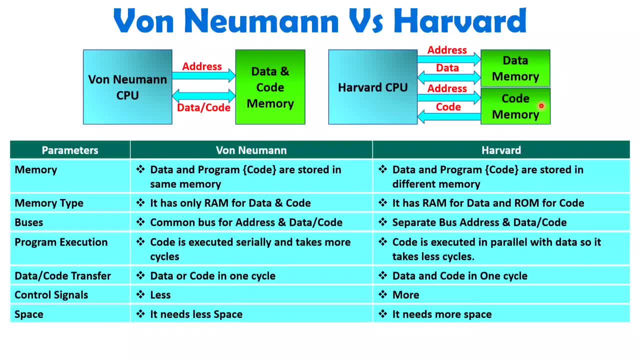 But with Harvard architecture, data and code memory is different, So in that case on board you will have to have more space Here. if you see what is the cost of this architecture, then obviously with single memory usage you need to have less cost. 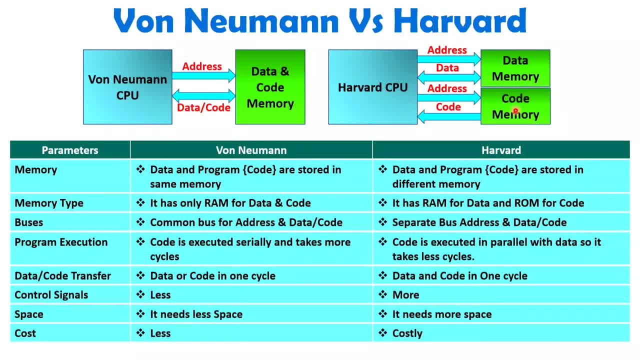 But with Harvard architecture it will be costly. It is not because of memory only, It is because of how we provide addressing, how we integrate our bus interface. so all those things in total makes system costly, right? So you can say: 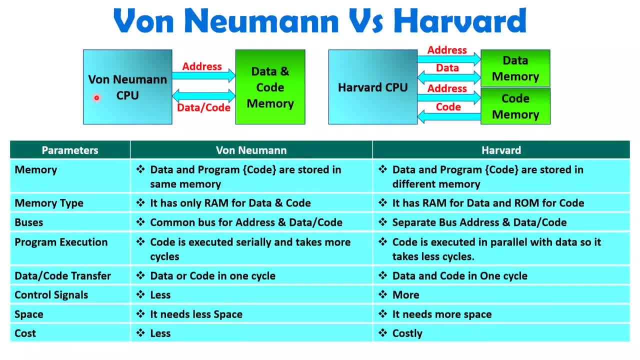 Harvard architecture is having better performance compared to one Newman. Why? The reason is Harvard is accessing data and code in parallel, While with one Newman you will have to have execution in serial manner with code and data. So Harvard is costly but efficient.